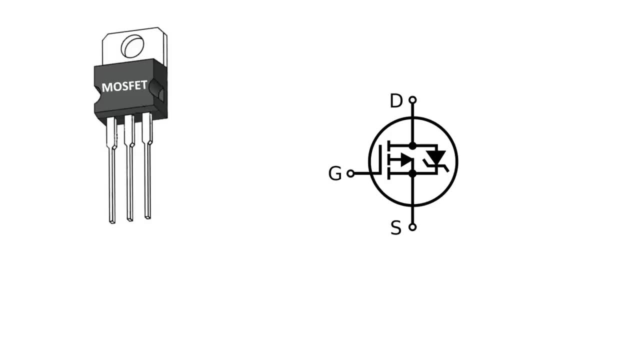 of a MOSFET transistor on the left and the symbol on the right. MOSFET also has three pins, As in JFET. one of them is gate, the other is drain and the last is source. Pin names are the same. 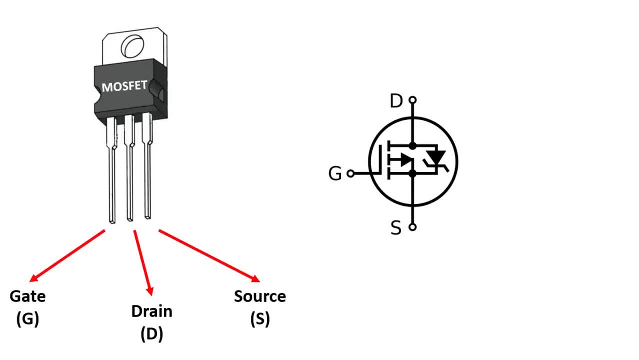 in MOSFET as in JFET. Their order is not always like this. Locations may vary depending on the model. G, D and S abbreviations are used for these In the symbol. the pin naming is like this: We can compare the structure of the MOSFET to a faucet. 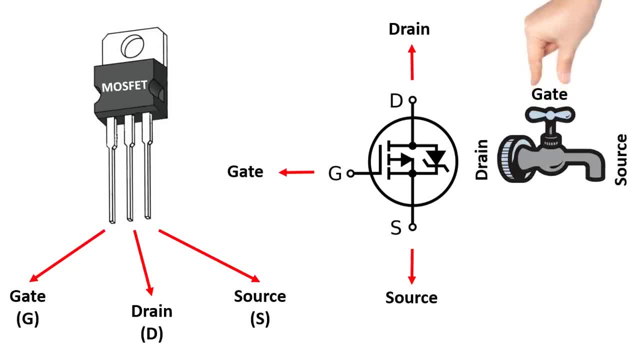 as in all transistors, We can think of the gate pin, where the trigger is made as the valve of the faucet and between the drain to source, where the current passes as the direction in which the water flows in the faucet When a trigger voltage is applied between 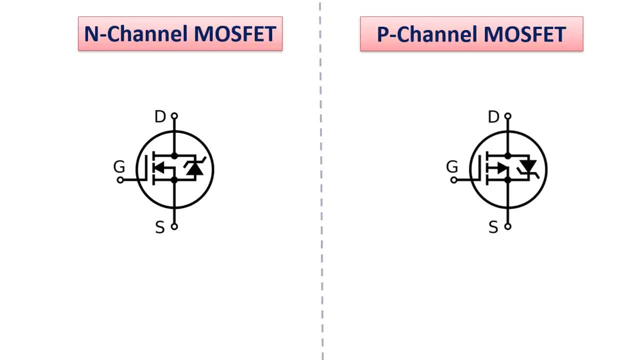 source, a current between drain and source is controlled. MOSFETs are produced in two ways: N-channel and P-channel. In the symbol, the outward arrow on the gate pin is N-channel and the inward one is P-channel. If you remember, it was the opposite in JFET. 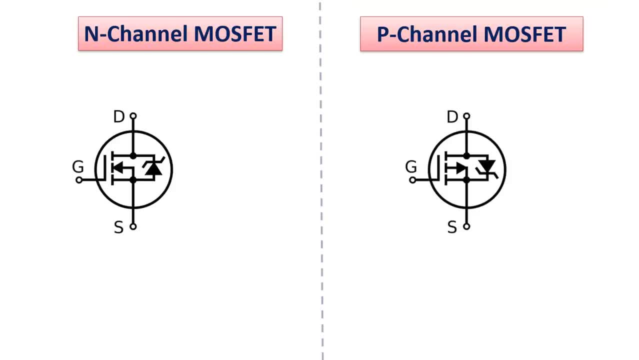 So what's the difference between them? The working principle of both is the same. The direction of the controlled current in N-channel MOSFET is from drain to source, while the direction of controlled current in P-channel MOSFET is from source to drain. In other words, 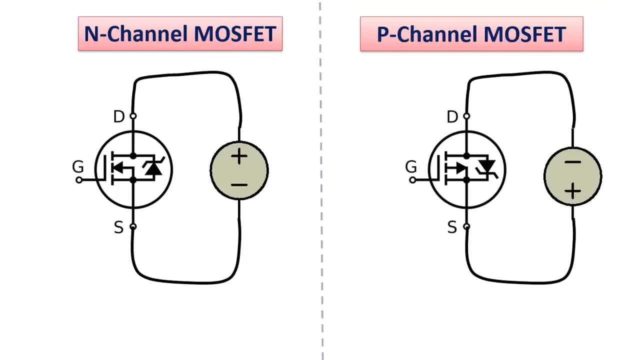 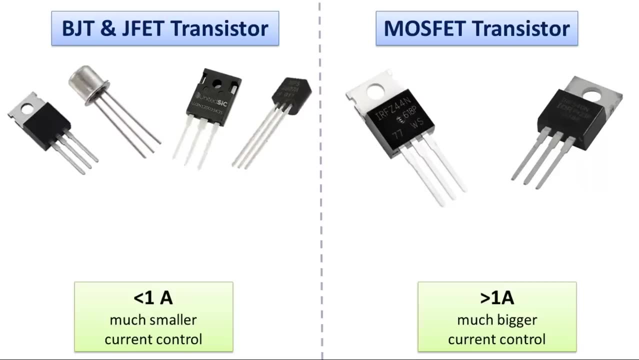 while the positive or plus pole of the voltage source is connected to the drain pin of the MOSFET in N-channel MOSFET, the positive or plus pole of the voltage source is connected to the source pin of the MOSFET in P-channel MOSFET. Let's compare MOSFET, BJT and JFET transistors. 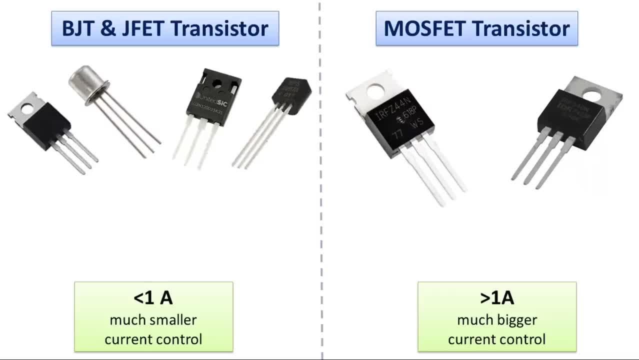 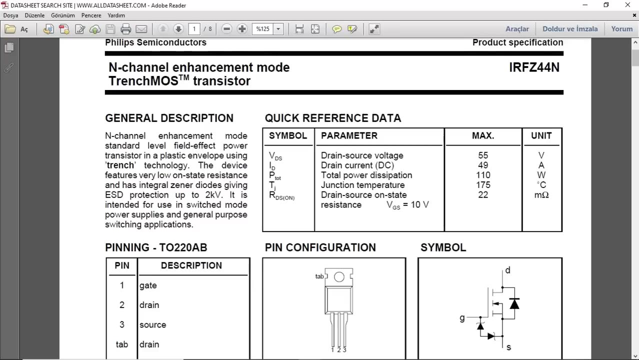 according to the current they can withstand. While currents close to 1 amp and under 1 amp can be controlled with BJT and JFET transistors, much larger currents can be controlled with MOSFET transistors. We can see this by looking at the datasheet of some MOSFET transistors. 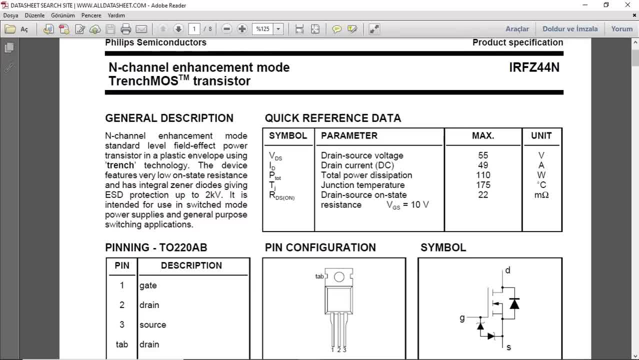 For example, when we look at the datasheet information of the very widely used IRF-Z44 MOSFET, there is information that current can be controlled up to a maximum current of 49 amps. This current value is really a great value. In addition, 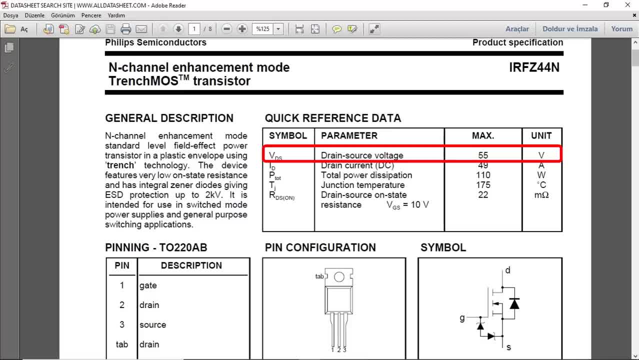 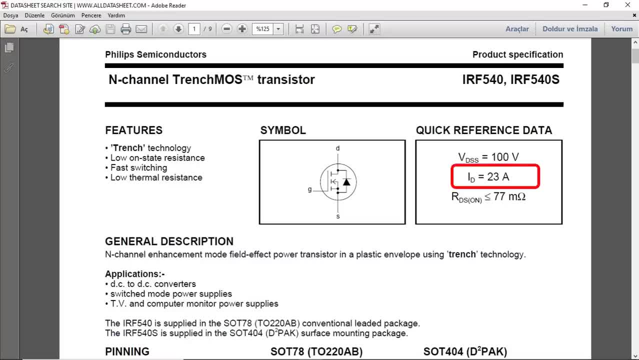 a voltage of 55 volts can be controlled with this MOSFET. When we look at the datasheet of IRF-540 MOSFET, another widely used MOSFET, there is information that a maximum current of 23 amps can be controlled. 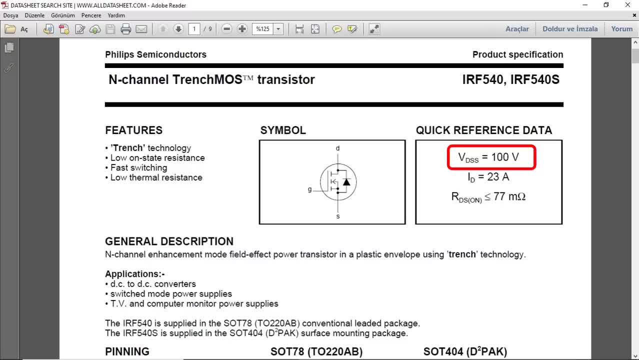 and a maximum voltage of 100 volts can be controlled with it. The fact that a wide range and much greater current and voltage control can be achieved with MOSFET increases the attractiveness of MOSFET compared to other transistors. For example, you see a. 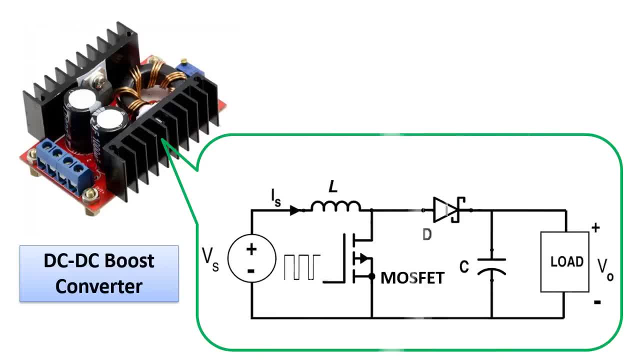 DC-to-DC boost converter. here The circuit diagram for this is basically the same as here. The amplification process is according to the switching speed of the MOSFET located here. Triggers are made at high frequency values at the kHz level In this way. 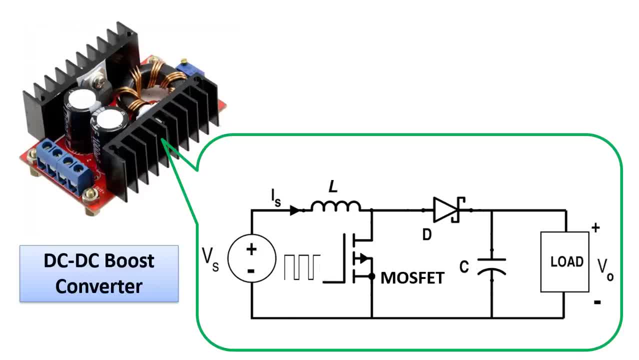 MOSFET and shock diodes are preferred in order to obtain healthier results, instead of using normal silicon diodes in order to respond to high frequency switching speeds in converter circuits, For example, you see a DC-to-DC boost converter here. The circuit diagram for this is basically the: 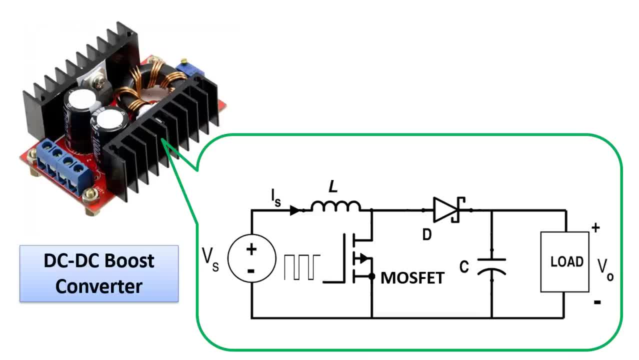 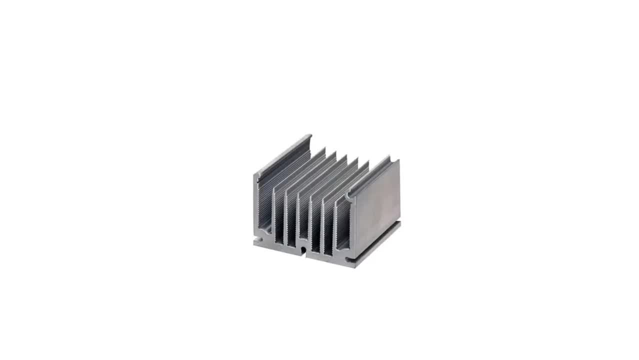 same as here. The amplification process is according to the switching speed of the MOSFET located here. dc converters and motor drivers using mosfets naturally get hot because very high current flows through them. as such, they need coolers. we usually see mosfets and circuits as fixed to heat sinks. 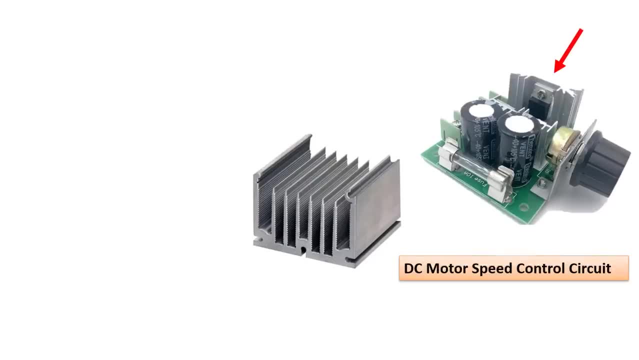 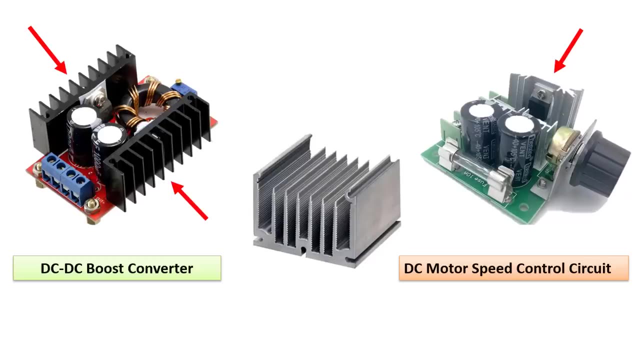 that will dissipate the heat, like you see here, for example, in the motor speed control circuit. you see, on the right here there is a heat sink fixed to the mosfet, which i show with the red arrow. we can see that there are heatsinks connected to mosfets in this dc to dc boost converter amplifier. 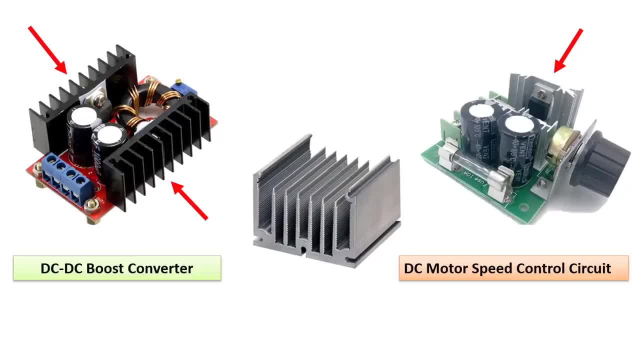 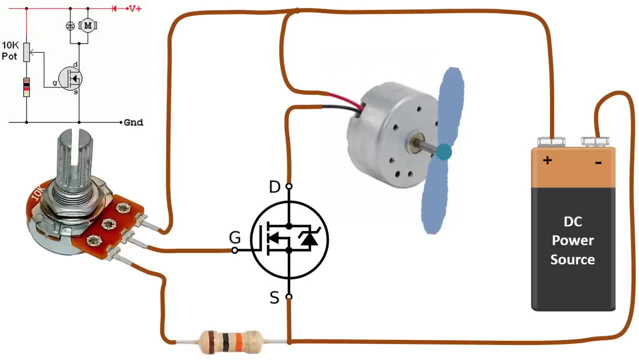 converter circuit you see on the left. well, let's look at the basic working principle of a mosfet. now, here you see a simple motor speed control circuit with the circuit diagram. in the upper left corner there is a small dc motor connected to the drain pin of the n-channel mosfet. 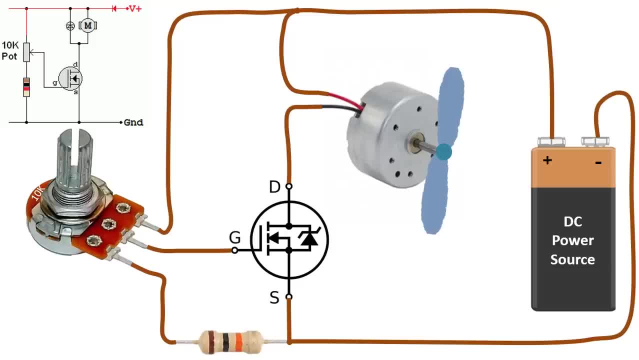 there is a dc source to drive this motor. here there is a potentiometer connected between the dc and the dc motors and the dc motor is connected to the dc source of the mosfet, the gate and source pins of the MOSFET, to provide the voltage to trigger the MOSFET. 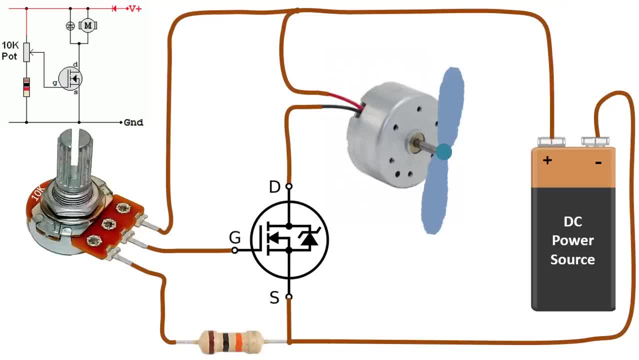 The reason for connecting a resistor between the potentiometer and the MOSFET is that a reverse current in the MOSFETs does not damage the circuit elements connected to the gate pin. Thanks to the resistor here, the intensity of that current is reduced. 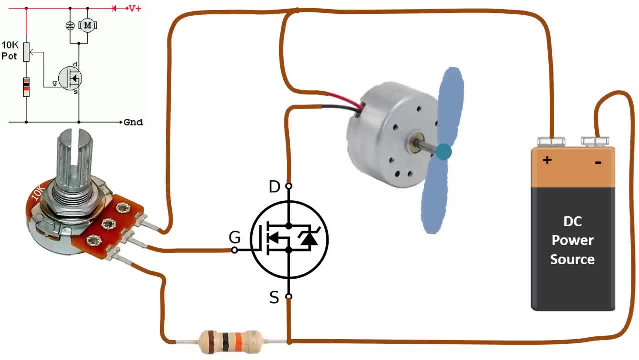 Thus, the circuit devices connected to the gate pin are not damaged If we talk about this circuit. since there is no damage to the potentiometer, this circuit will work smoothly even if there is no resistor. Now, when we change the resistance value of the potentiometer here, 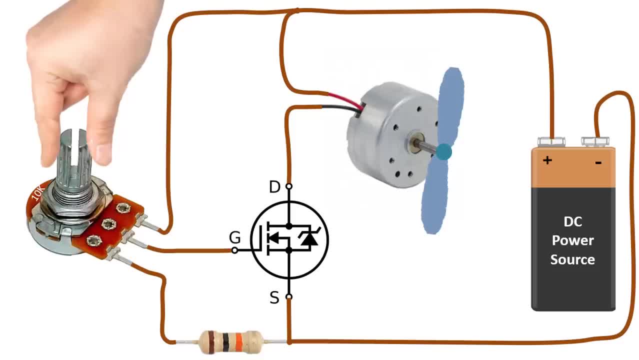 a voltage will be applied between the gate and source of the MOSFET. With this voltage, the MOSFET will be triggered and the current coming out of the positive or plus pole of our power supply will flow between the drain and source pins of the MOSFET by. 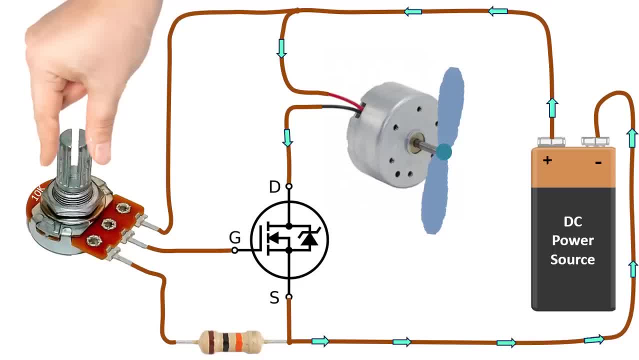 following the path we have shown with the arrows, and our motor will rotate with this current. As the trigger voltage will change by increasing or decreasing the resistance value of the potentiometer, the drain current will change and the speed of the motor will change according to. 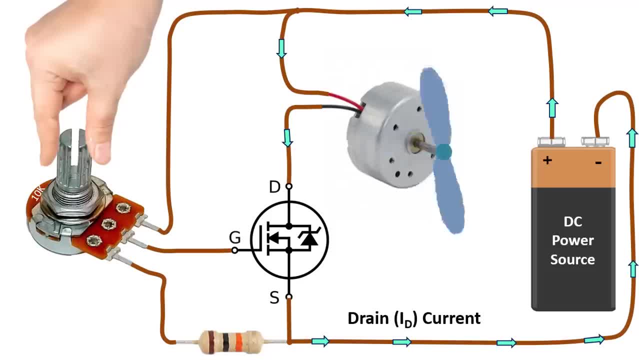 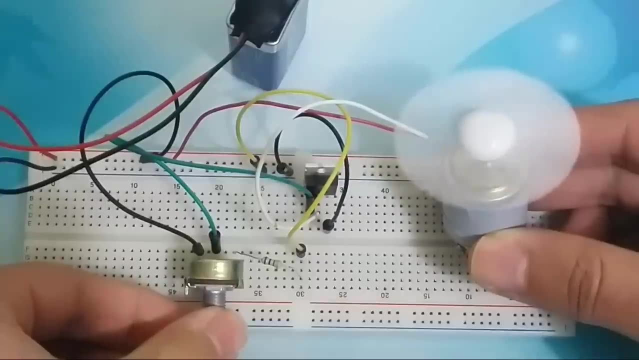 this current. We can also control the motor by connecting a power supply that provides a constant 5-volt voltage instead of a potentiometer. While the MOSFET is triggered above 5 volts, it is not triggered at the voltage below. For a better understanding of this, motor speed control: 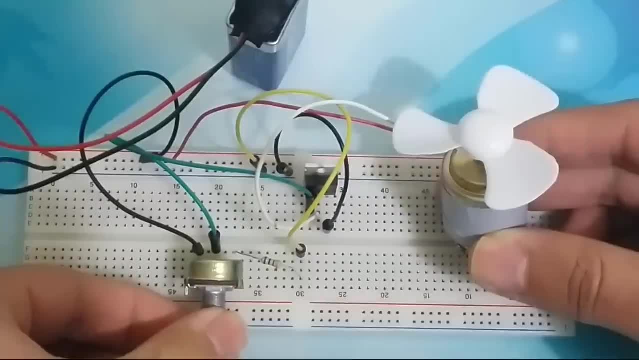 circuit. I built the circuit on a breadboard. As you can see, the motor is connected to the board With a 9-volt battery. we can control the speed of a small DC motor with a potentiometer thanks to the MOSFET. in this way, As here, the working principle of systems with big electric. 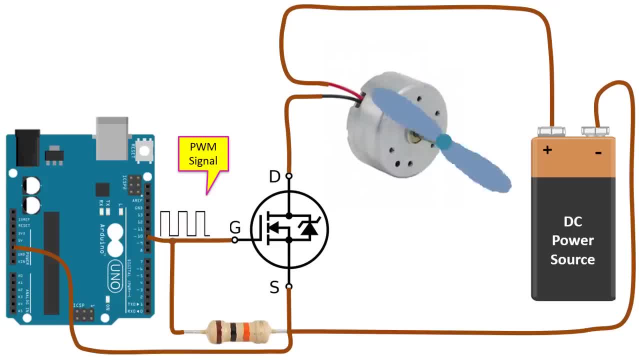 motor fans is the same. With MOSFET, we can control the speed of a motor not only with a potentiometer, but also with a microcontroller, as here. Since the resistance value on the gate pin of the MOSFET transistors is very large, there is no current flow. 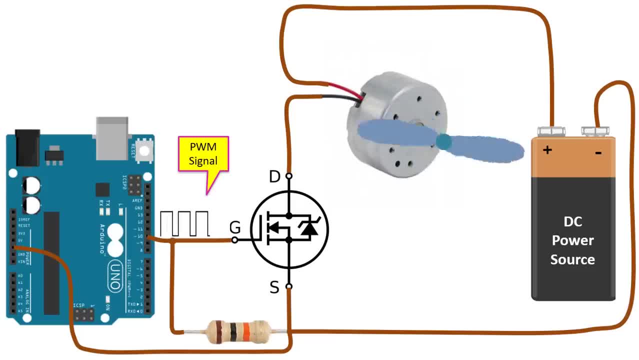 That is, the trigger part and the part connected to the load are isolated from each other. As such, MOSFET can be easily used with a microcontroller such as Arduino, Thanks to the 5-volt square wave received from the PWM signal output of the Arduino. 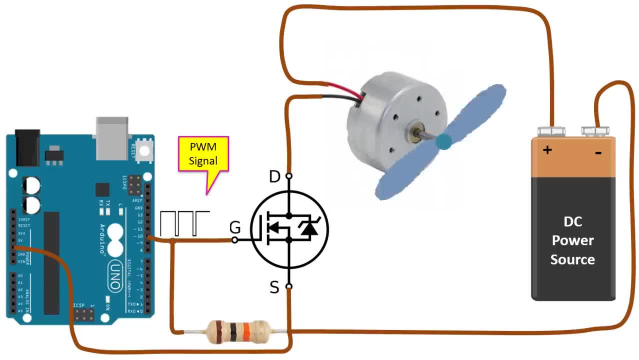 speed control can be done easily According to the duty value of this signal, that is, by adjusting the expansion and contraction of the signal. we can make the motor rotate fast or slow. Here the resistor connected to the source pin of the MOSFET provides protection for the reverse current that may come to the Arduino.